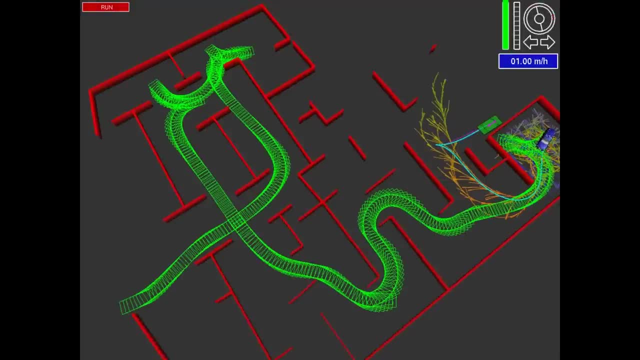 path to the goal, And that's what we're going to see in this video. When you implement this yourself, the big difference to our grid implementation is a different motion model. You have to implement a robot that is able to turn and you have to. 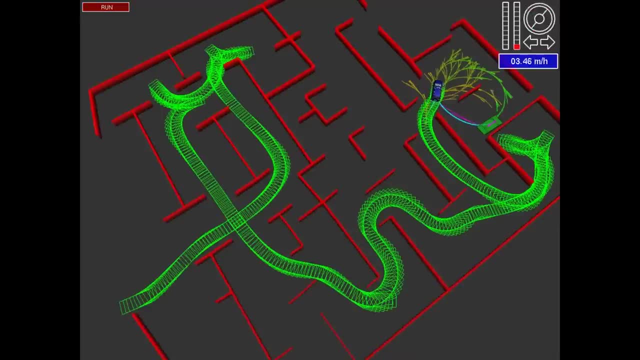 write on the math of a robot that's able to turn and go forward. This robot also can revert, So going backwards is a discrete different action, But other than that, it's essentially the same A-star algorithm you just implemented. So if you want to build a self-driving car, 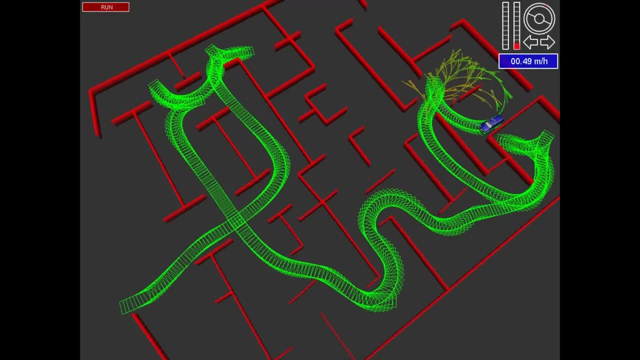 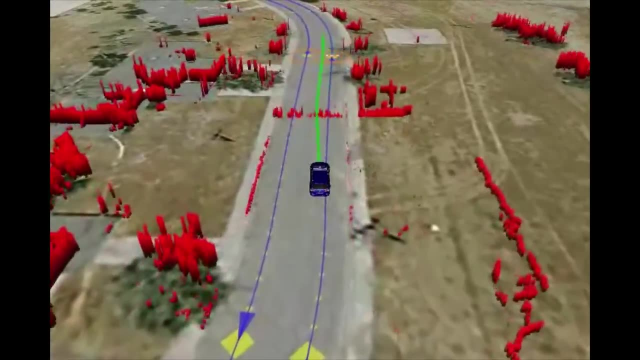 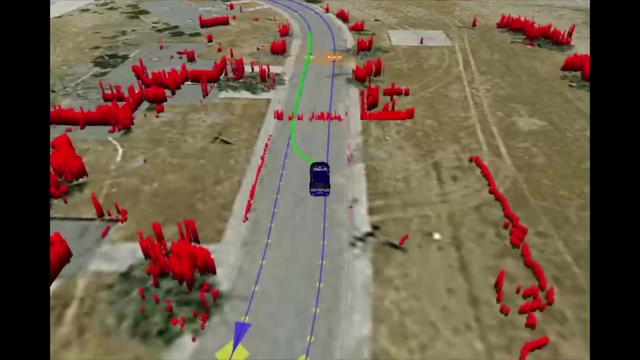 you know, I understand to make a really complex, nice search algorithm to find a path to a goal. So this is a scene where DARPA trapped our car using a barrier that went all across the street. So the only way for the car to navigate this was to take a multi-pole U-turn, and it had to plan. 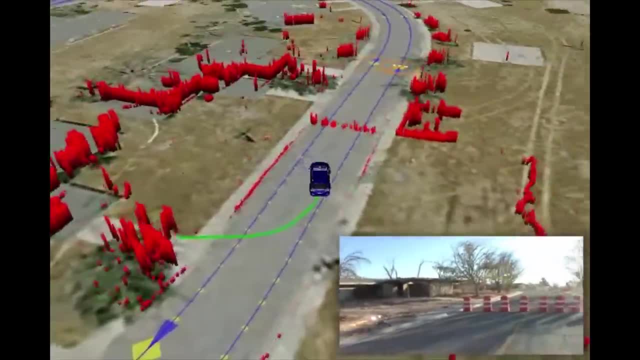 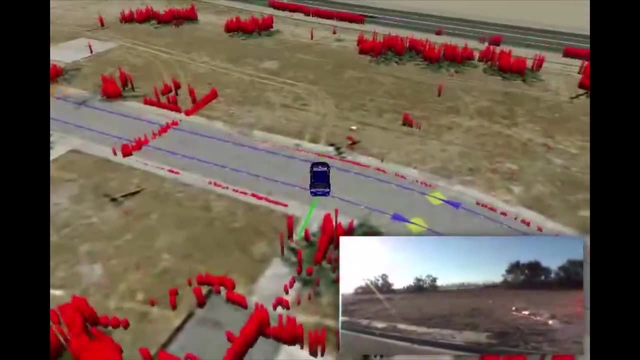 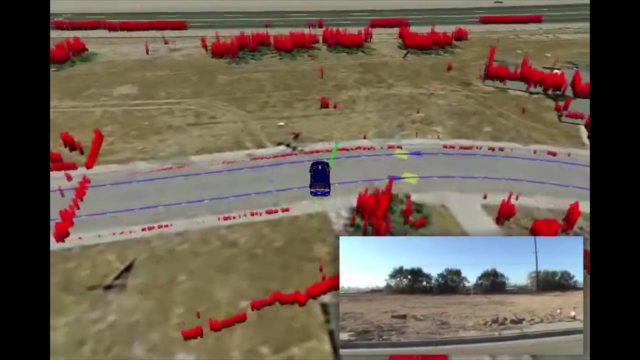 this all by itself, using A-star planning. The car pulls up to the barrier, realizes there's no path to go, then invokes its A-star planner and comes up with a turnaround maneuver that is not particularly elegant, but it's super effective And the car was able, in this competition, by itself, to turn around. 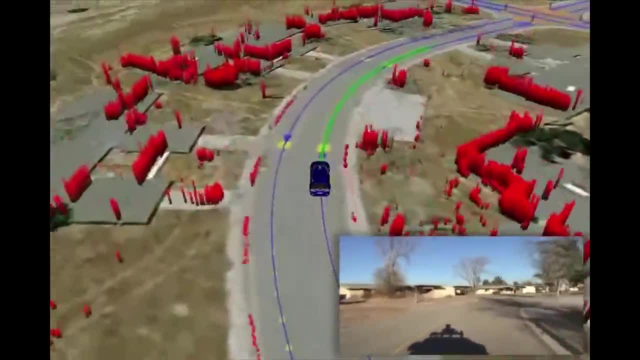 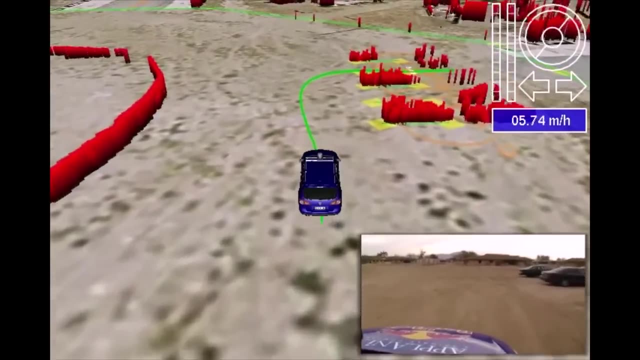 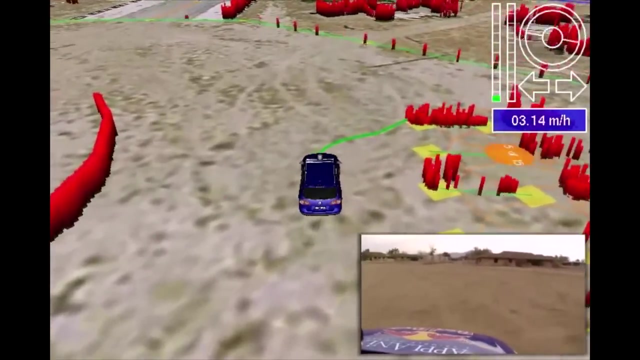 using A-star, find the optimal plan to do so and move on. Otherwise, it would have been stuck forever behind this obstacle. In this final video, I show you a parking situation where the car has to back into a parking space between two other cars, and you can see how the obstacles are. 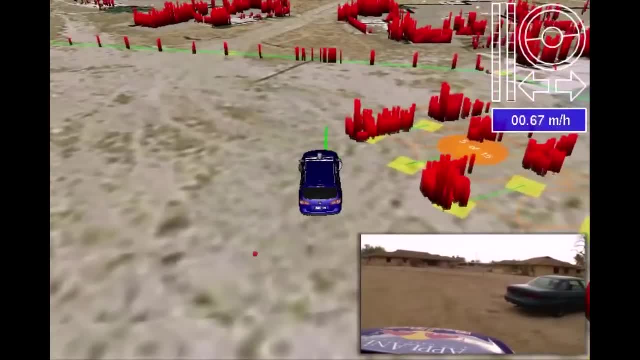 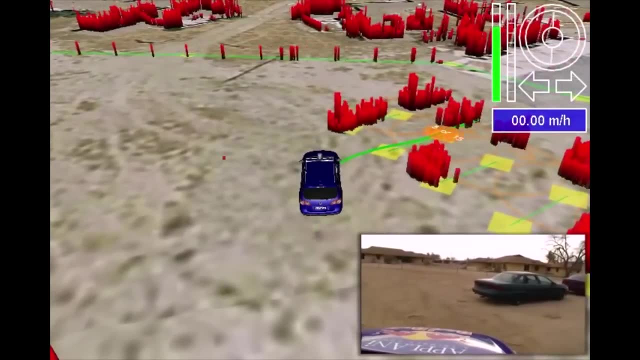 visible, how these other cars are visible and how our vehicle junior navigates an actual parking lot. Again, this is using A-star. It finds its way optimally into this parking spot, backs in and backs out again. all by itself, The planning time for each of these A-star runs is less than 10 milliseconds. 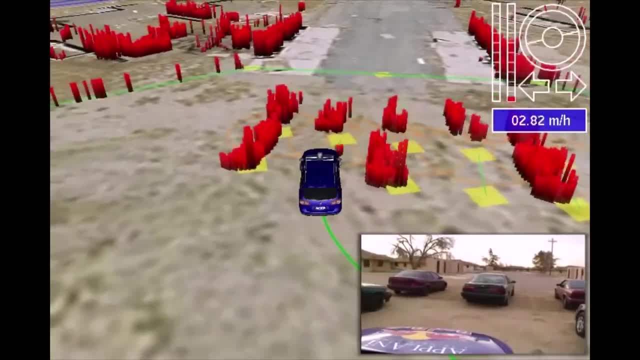 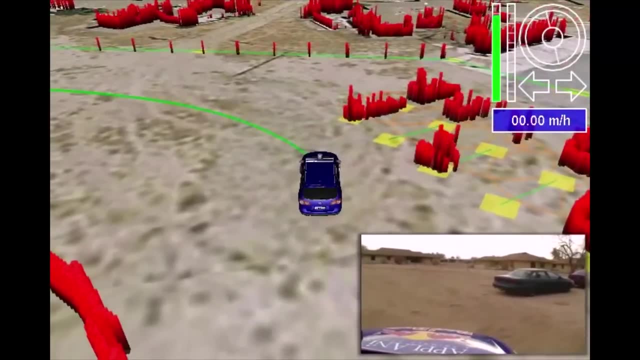 and the car was able to competently do this even though in advance, it had no clue where the obstacles were and where the parking spot was. That is A-star for robot path planning, And what you've implemented yourself is the core of it. Again, if you want to turn it into a real robotic, 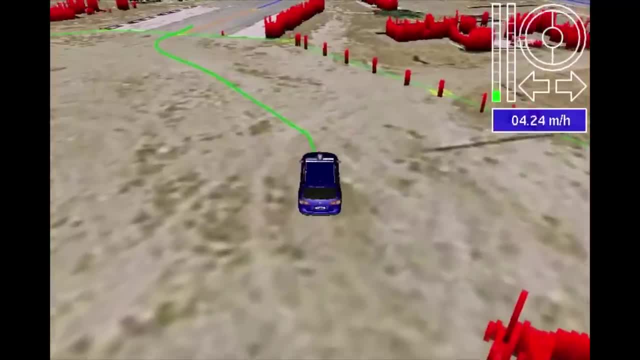 motion algorithm. you can do that by using A-star, And that's what we're going to do. You have to change the motion model and you have to see the next class I'm teaching you when I go to continuous values and show how to turn this into a continuous motion path.